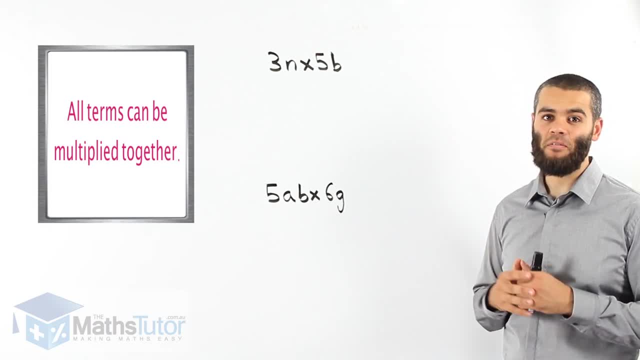 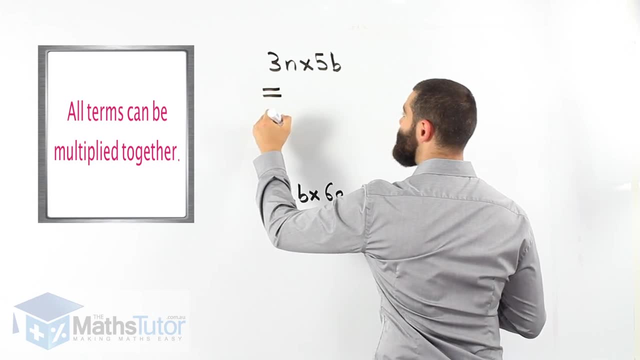 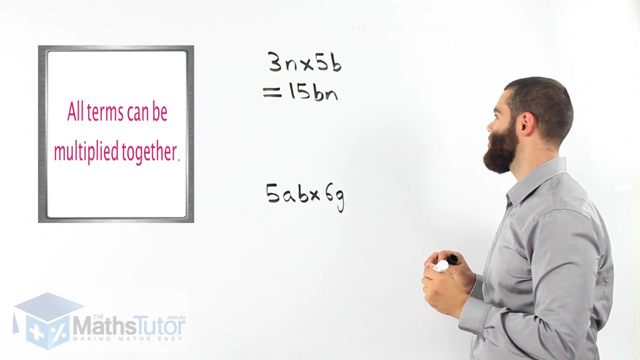 we don't worry about like terms With multiplication, it doesn't matter. So 3n times 5b, Simple, We know our times tables. 3 times 5 is 15bn or nb, but it's better to put in alphabetical order. So 3 times 5, 15bn, It's. 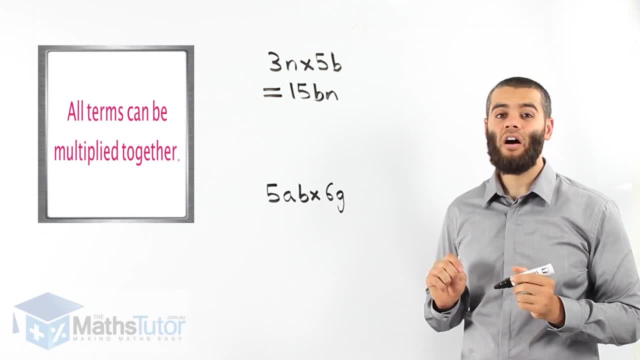 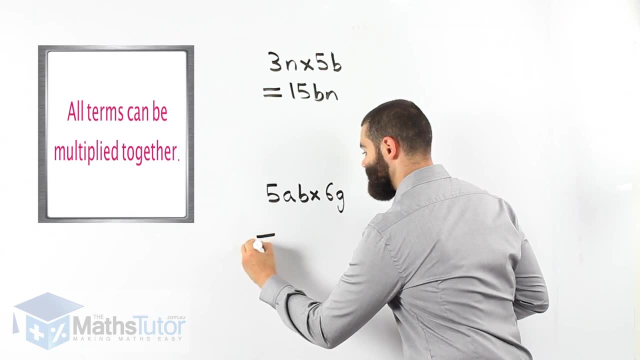 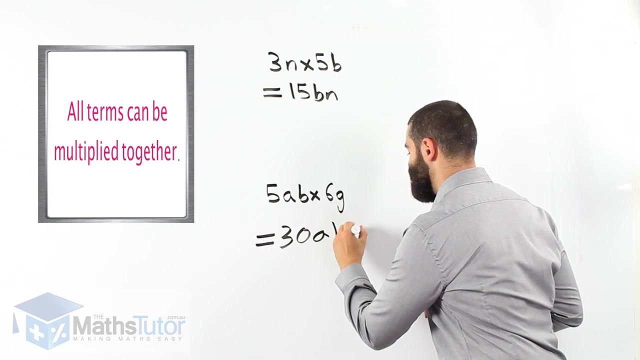 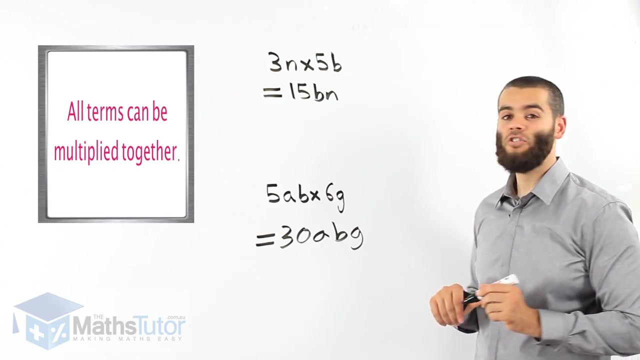 that easy Here. 5ab times 6g. Again, we just multiply the numbers 5 times 6, 30. And we don't get abs. G are our pronumerals ab and g. So 5 times 6, 30abg. Now let's do another 2 more. 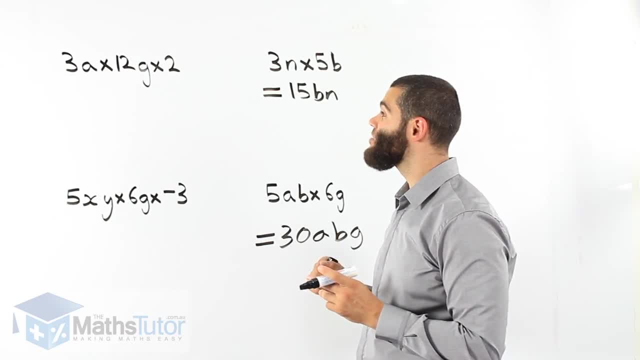 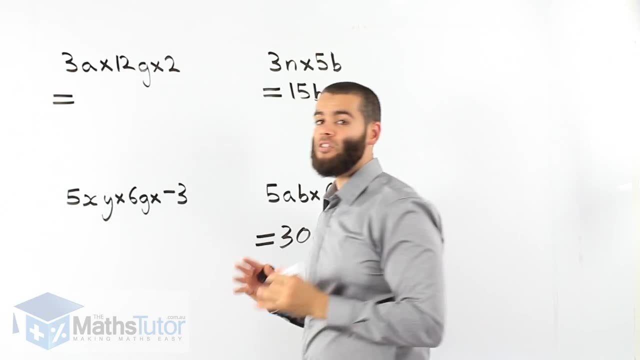 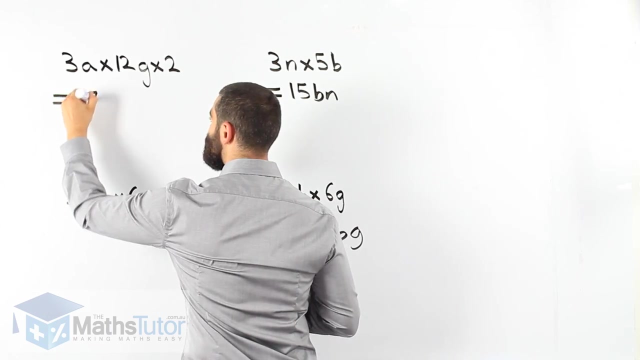 We have 3a times 12g times 2.. Again, we multiply everything 3 times 12,, 36.. 3 times 12,, 36.. 36 times 2, 70.. 72 a g. 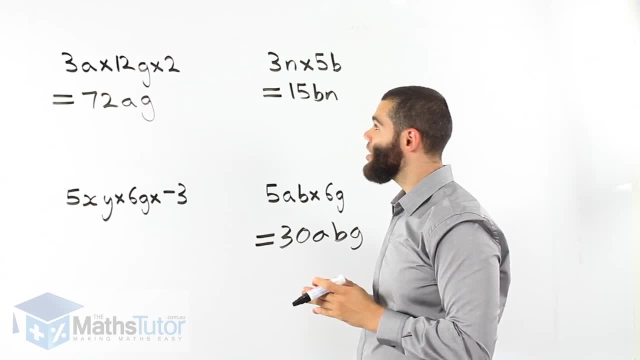 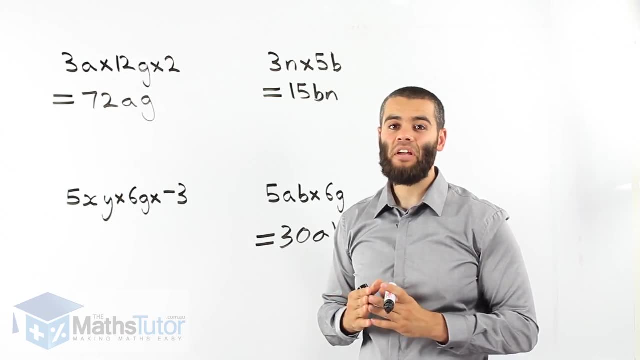 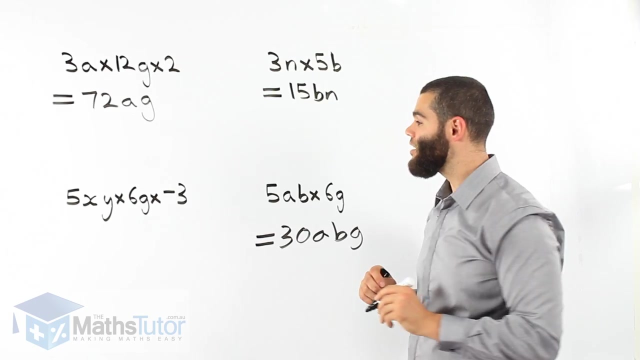 So 3 times 12 is 36, times 2 is 72. Again, we put the pronumerals a g. There they are, We put them in our answer. our final answer: 72 a g. Now we have 5xy times, 6g times, negative 3.. 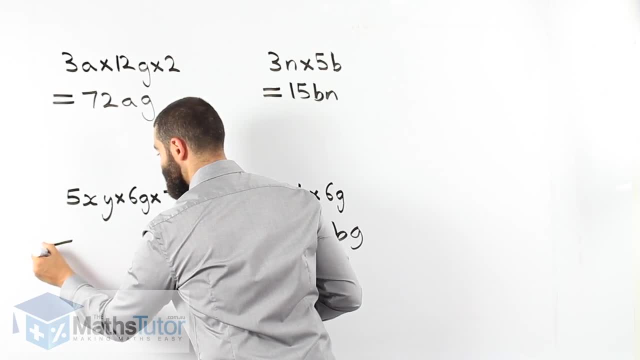 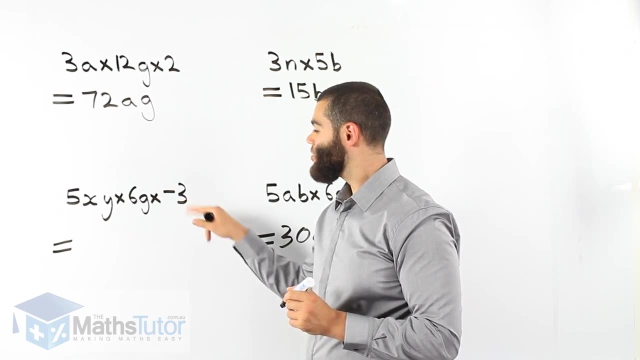 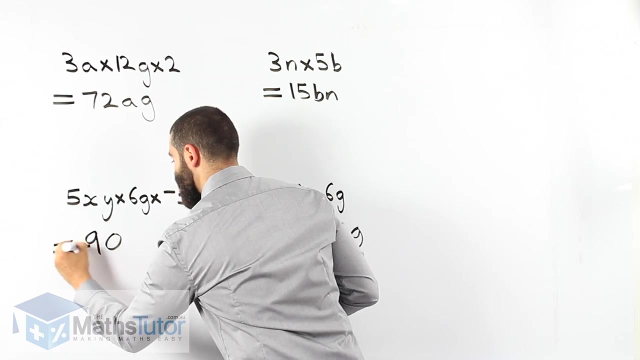 We multiply the numbers, So 5 times 6 is 30,, then 30 times negative 3.. So we know that 30 times 3 is 90, and we put our negative. So 5 times 6 is 30.. 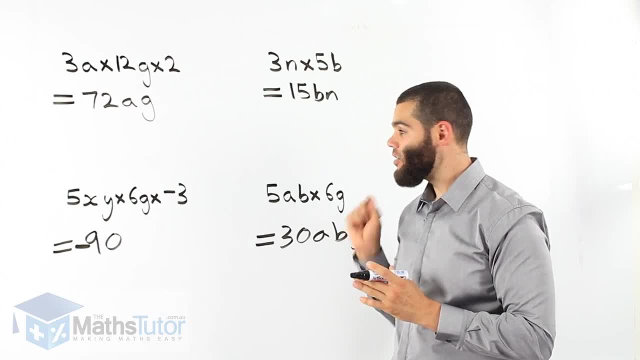 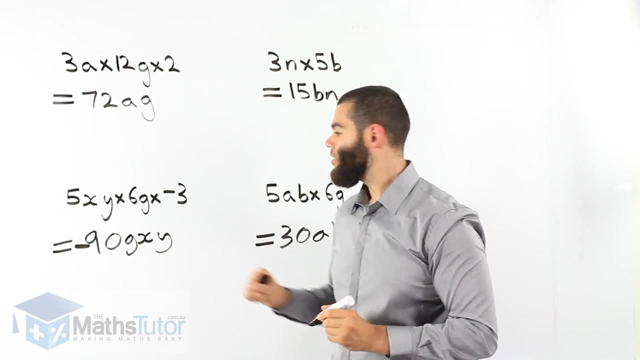 30 times negative. 3 is negative 90. Don't forget the negative. And of course we can write it down as gxy. You can write the letters in any order or the pronumerals In any order, as long as you write them all down. 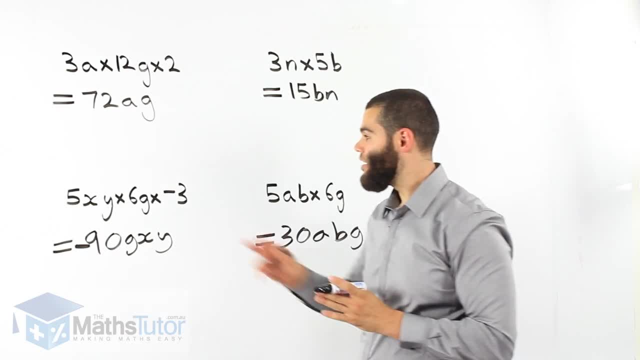 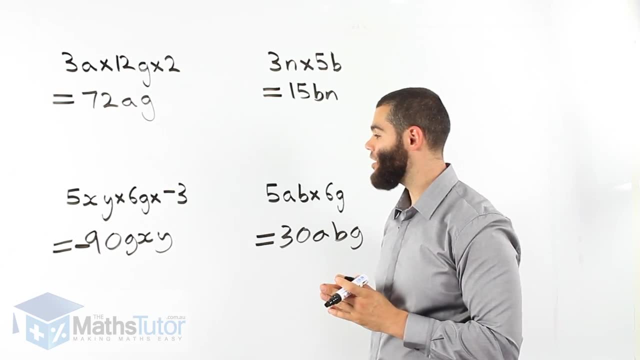 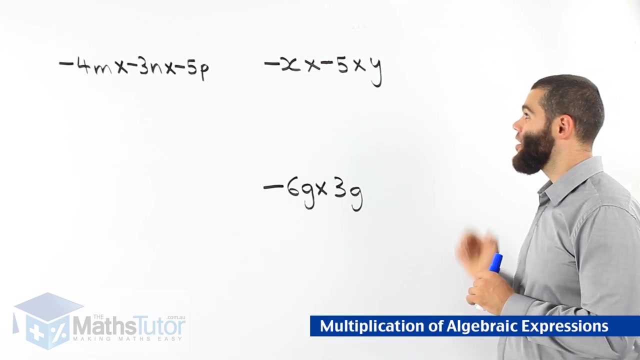 gxy or xyg, it doesn't matter. 5 times 6 is 30.. 30 times negative: 3 is negative 90.. Negative 90 gxy is our final answer. Okay, guys, last three examples: We have negative x times negative, 5 times y. 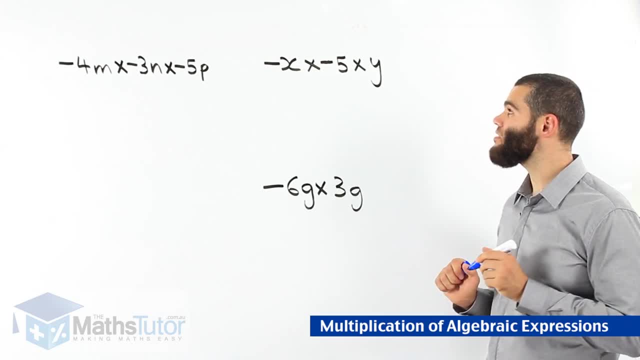 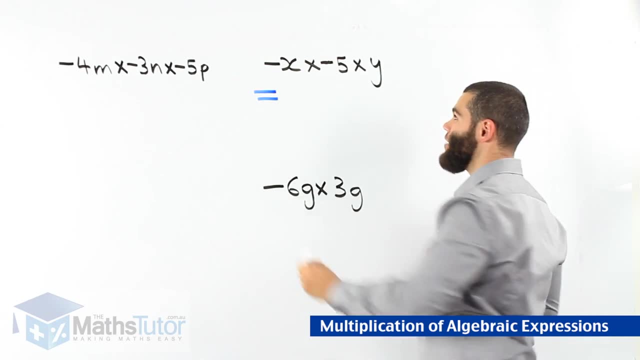 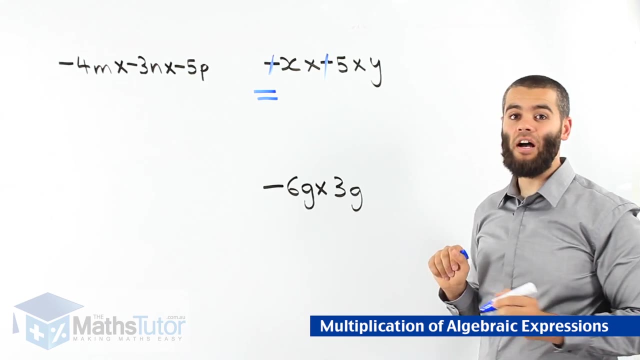 Well, same rules apply: Negative x times negative 5 times y. We know that negative x times negative 5, when we have two negatives, we cancel them out. They are gone. So 5 or x times 5 is 5x. 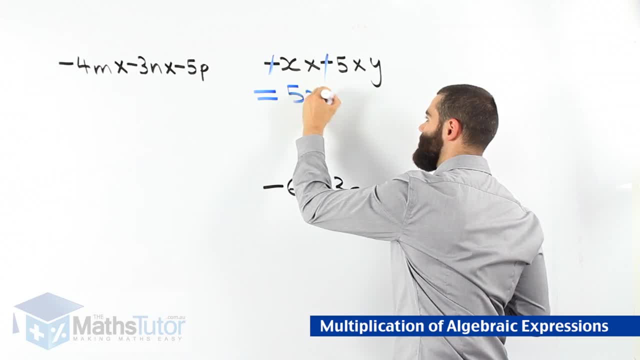 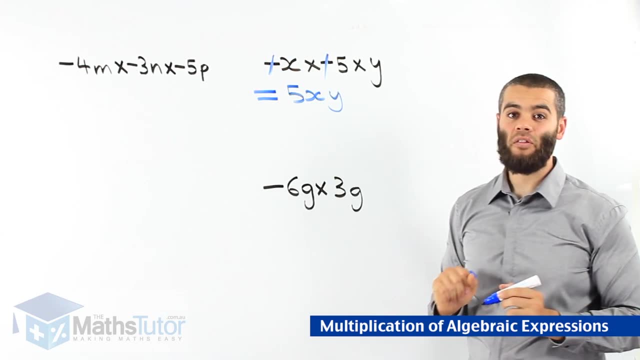 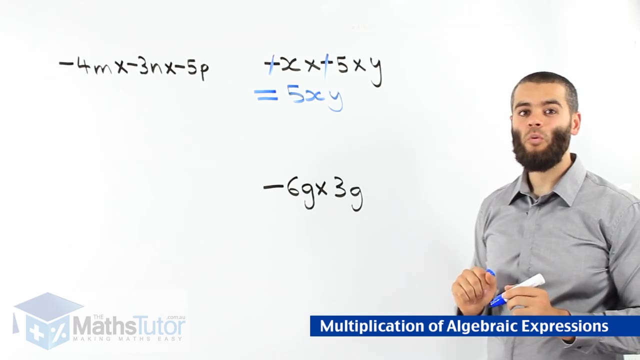 5x times y, 5xy. So negative x times negative 5 times y. The two negatives cancel each other out in multiplication. So x times 5 is 5x times y, 5xy. Here we have negative 6g times 3g. 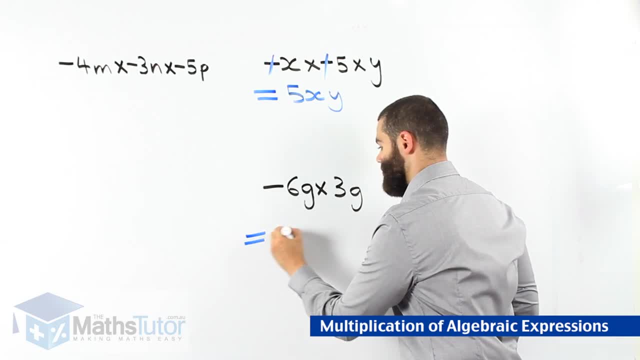 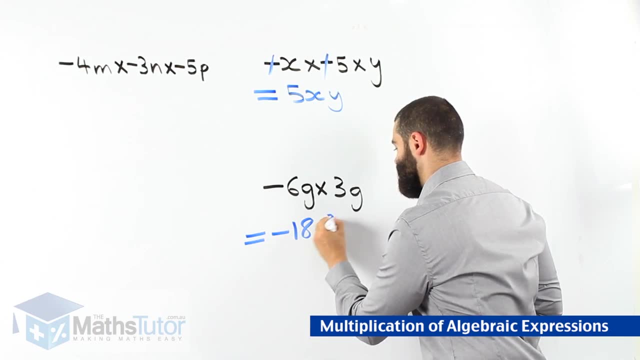 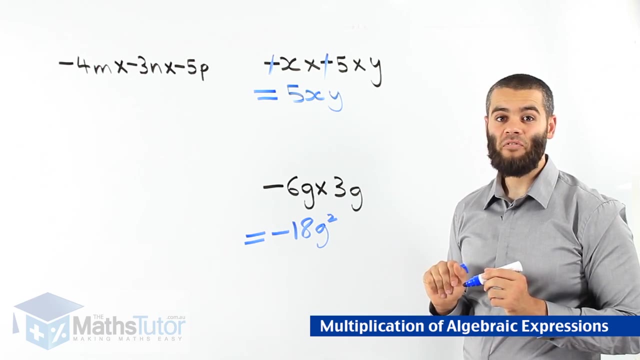 Negative. 6 times 3, negative 18.. And we know: g times g is g squared. Very important in multiplication: g times g is g squared. It's like saying 5 times 5, 5 squared, Or 10 times 10, 10 squared. 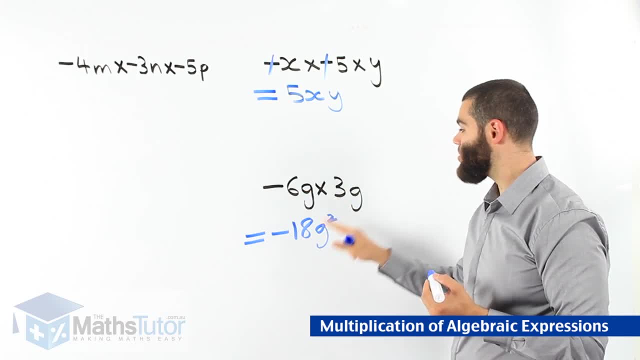 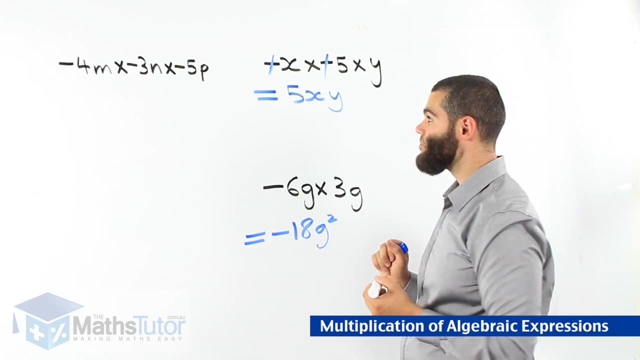 Very important multiplication that you realize that Negative 6 times 3 is negative 18.. g times g is g squared. Last example: Negative 4m times negative, 3n times negative: 5p. Well, let's get started with the multiplication. 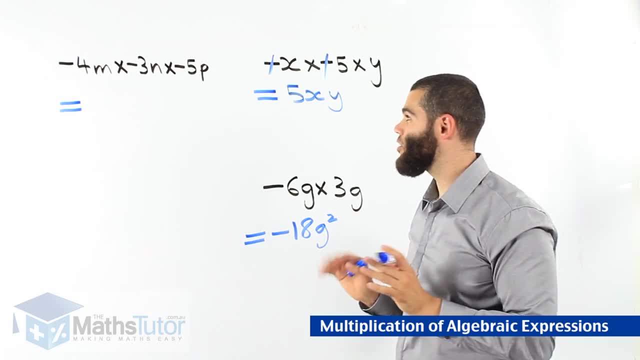 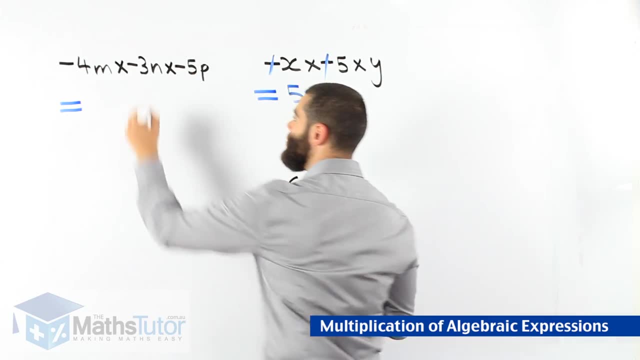 We know we multiply everything together. We don't look for like terms at all, We look for multiplication. You times everything together: Negative 4 times negative 3.. We know that they cancel. So 4 times 3 is 12.. 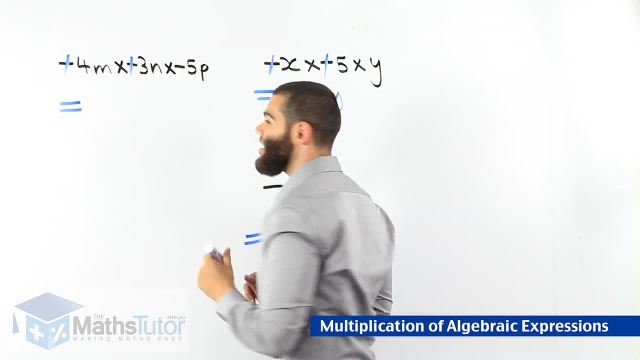 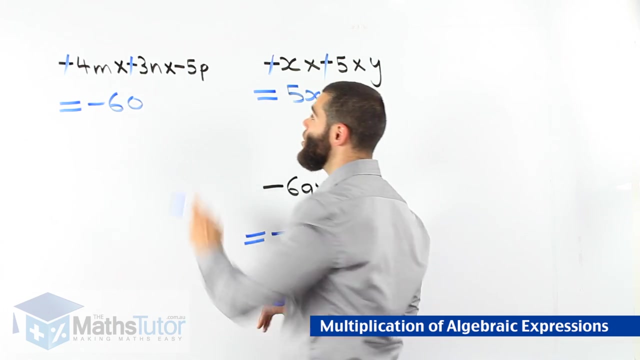 Then 12 times negative: 5.. So 12 times negative: 5 is negative 60.. So negative 4 times negative: 3.. The two negatives cancel 4 times 3 is 12.. 12 times negative: 5 is negative: 60..